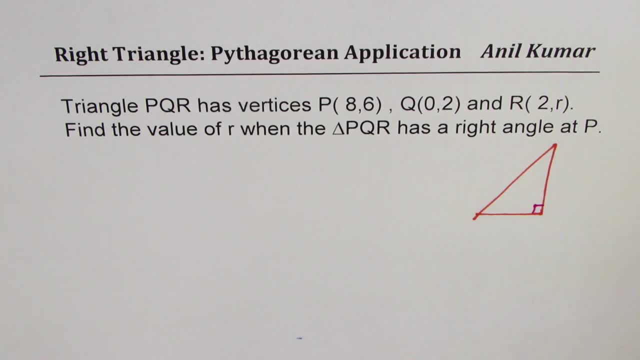 Coordinates given to us are: for P it is 86. for Q it is- let us say this right- Q. here we have 0 to and for our it is to our. okay, so this is an approximate drawing which helps you to just solve the question. we are not user. 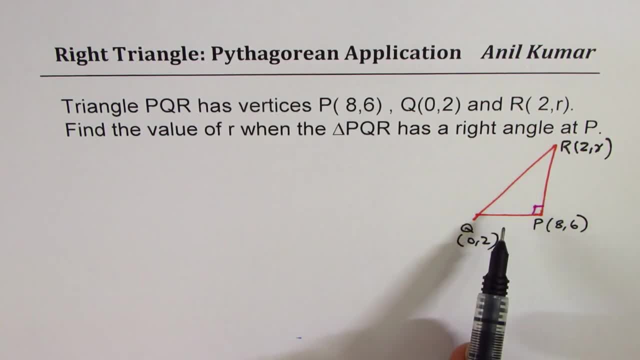 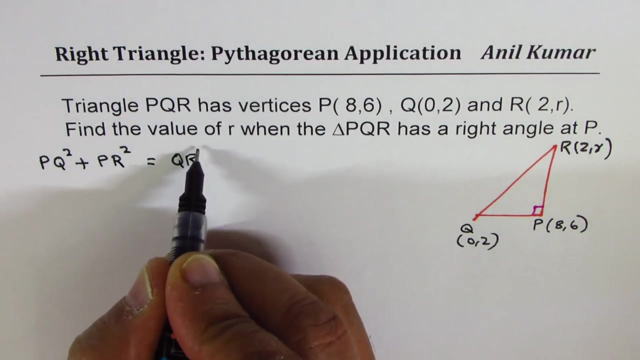 coordinate plane at all to place them properly now in a right triangle. you know, sum of squares of the smaller sides is equal to the square of hypotenuse. so we can write down our equation as: pq square plus pr square equals to qr square right. so that's the pythagorean theorem. 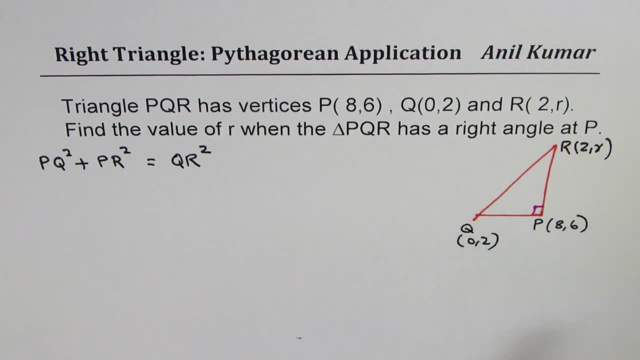 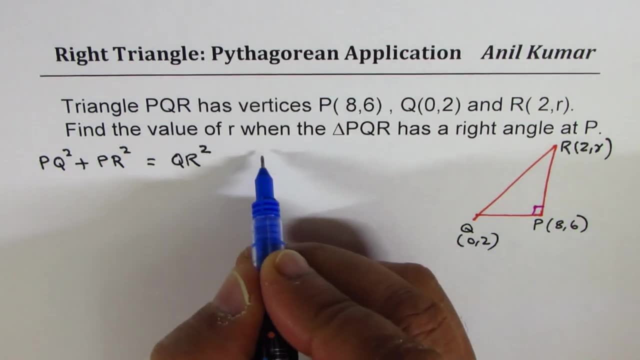 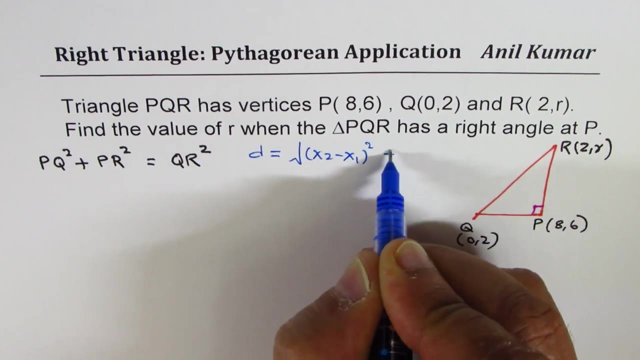 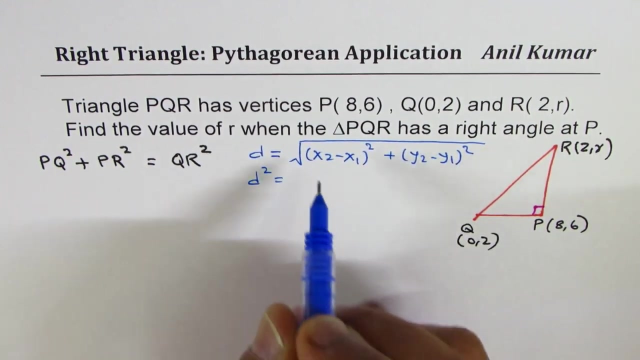 now to find the distance PQ, we will use the formula which is the distance formula. so as a reminder let me write down distance formula here as square root of X 2 minus X 1 whole square, plus Y 2 minus Y 1 whole squared. and when I square then we get rid of the square root, we get X 2. 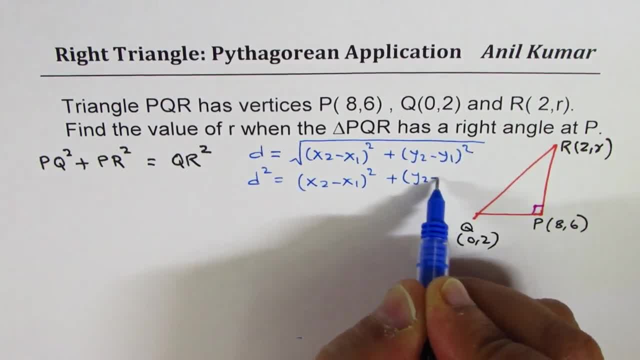 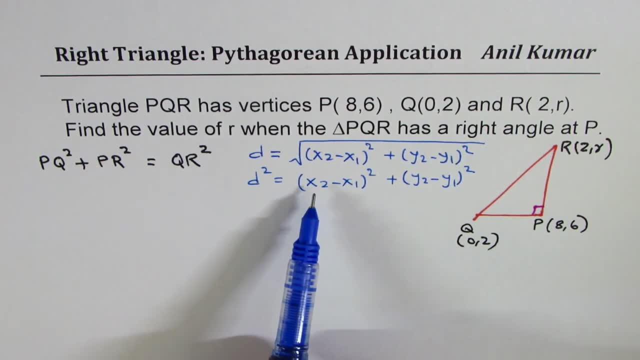 minus X: 1 whole square, plus y2 minus y1 whole square. Now you may also need the formula for x2 minus x1 whole square, since we are using a variable here, right? So let me write another formula which will be of use to us. 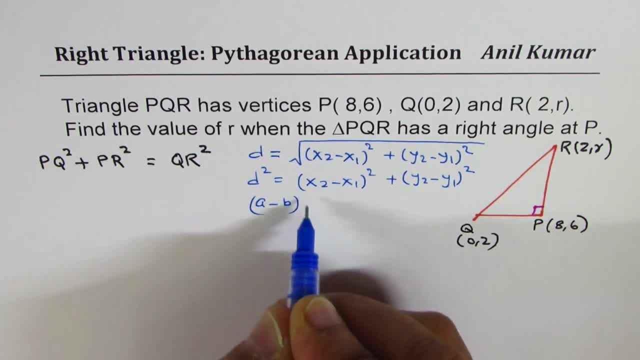 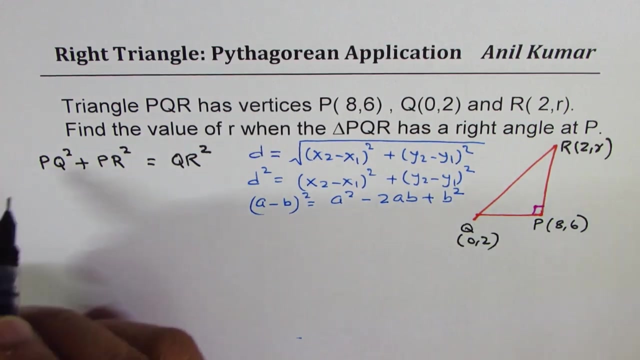 that we could write like a minus b, whole square will be a square minus 2ab plus b square. Now, with most of the things already explained, I would like you to pause the video and answer this question. okay, Now let's find out all these sides. so P cube, rather PQ square, is going to be. 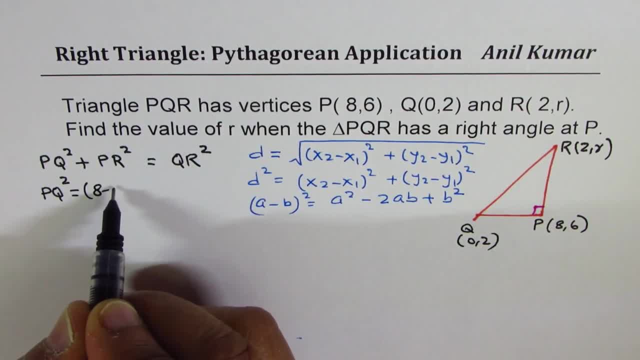 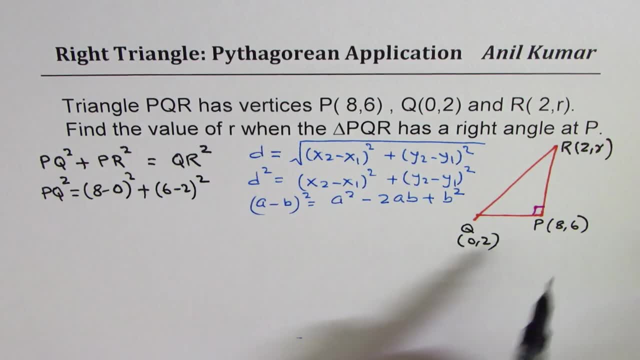 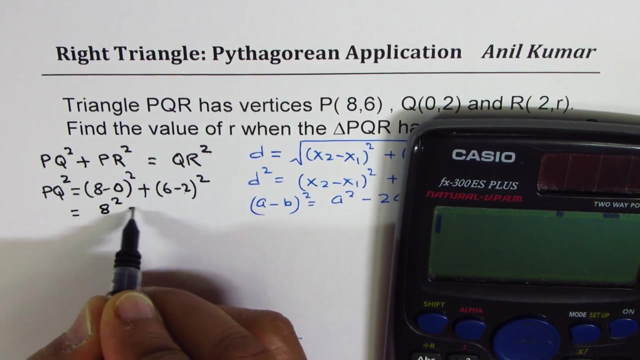 8 minus 2, 8 minus zero, I'm sorry- plus square plus 6 minus 2, whole square. right Now that gives us 64, 8 square plus 4 square. So what you can do is you can use calculator, right? So let me rewrite this: 8 square plus 6 minus 2 is 4, 4 square. 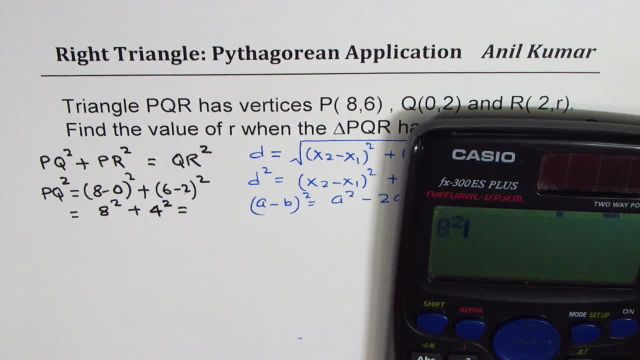 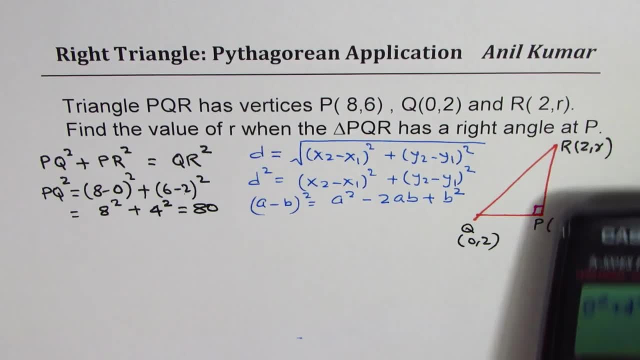 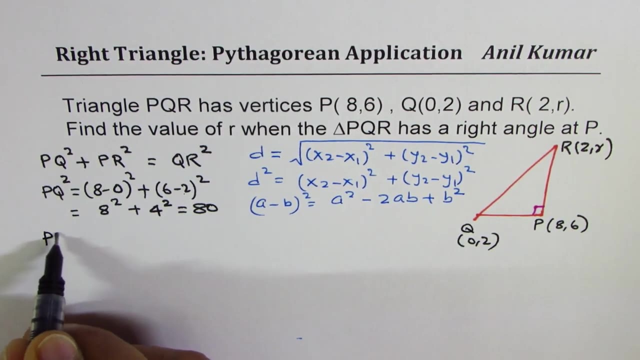 64 plus 16, right. So let's do: 8 square plus 4 square equals to 80.. So we get the length square of PQ. Now let's find what PR is. PR square will calculate. PR square will be 8 minus 2, whole square, plus 6 minus R, whole square. Now 8 minus 2 is 6.. 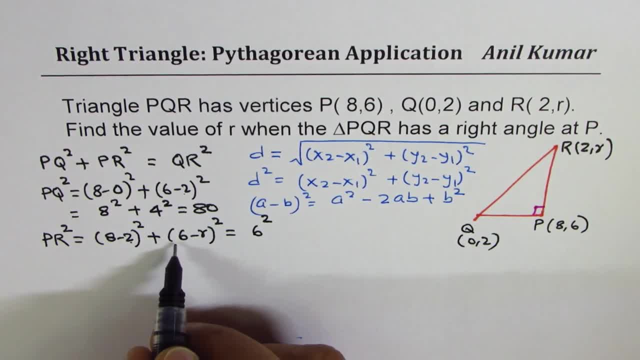 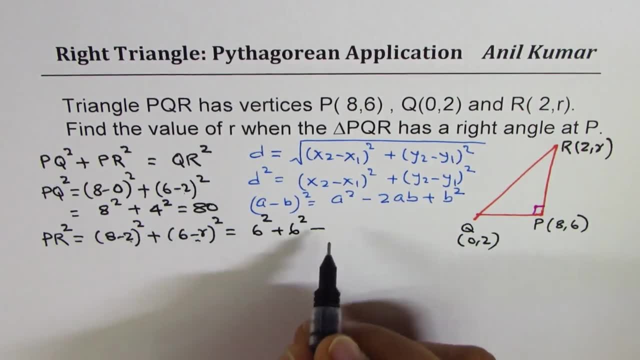 We can write 6 square and let us expand 6 minus R whole square using this formula: Right, So we get plus 6 square. minus 2 times 6 is 12 R and plus R square. So that gives us 36,. 36 is 72.. So we can write this as: let's write down here: So we get 72 minus. 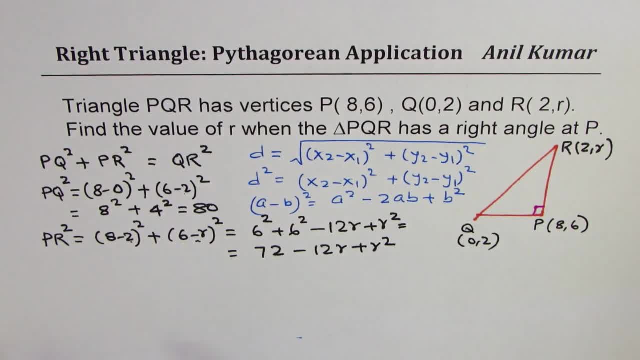 12: R plus R square. Okay, So that is PR square. What is QR square? QR square will be equal to 2 minus zero whole square, plus R minus 2 whole square. R minus 2 whole square. that gives us 2 square plus again. apply this formula, We get R square. 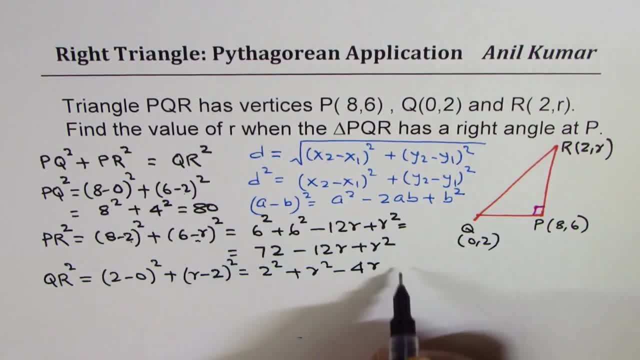 minus 2 AB, which is 4 R plus 2 square. So that gives us 4 plus 4 is 8.. And we have plus R square minus 2 AB, which is plus 5 R plus 4 into 3 or 16 minus 5 minus 4.. So that is. 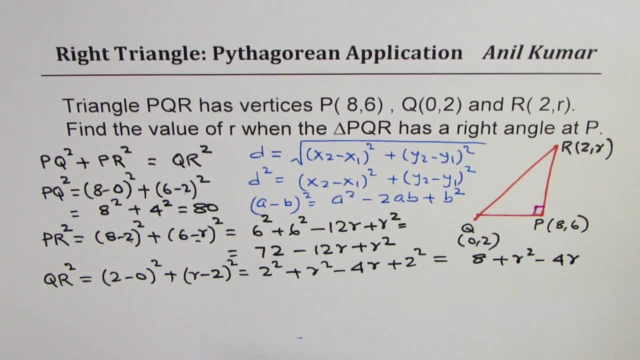 equal to 2 AAB plus 2 minus 2 square. 3 minus 2 square. Now we find R square이고 And that's minus 4R. Now we are going to substitute these three values into our first equation, right. 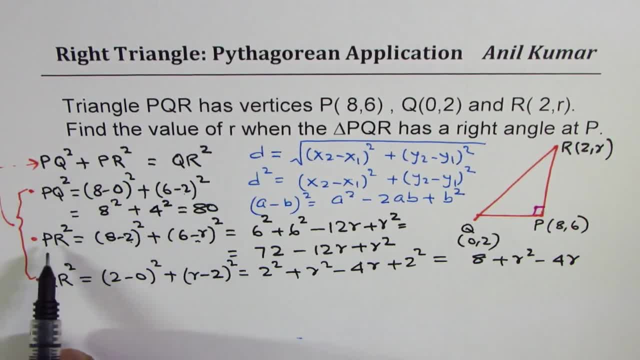 which is Pythagorean theorem. PQ square plus PR square means 80 plus PR square is 72 minus 12R. plus R square is equal to QR square, which is 8 plus R square minus 4R. Now we can bring the 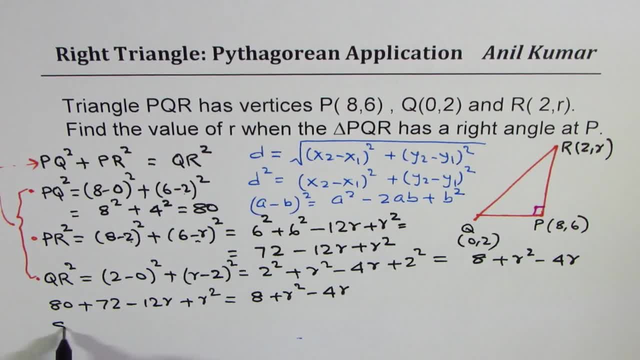 variables on one side and constants on the other side. So we get 80 plus 72 minus 8 equals to R square minus 4R, 4R minus R square plus 12R, correct, Okay? So let's solve this equation: R square minus R. 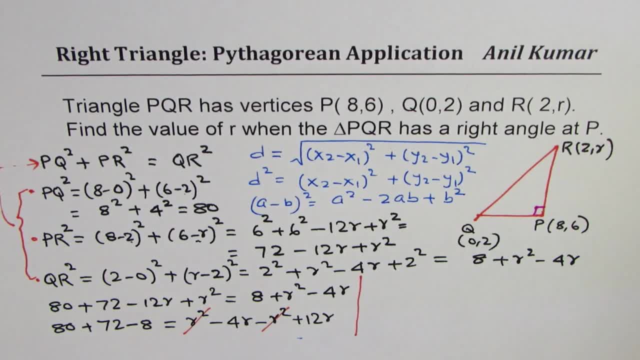 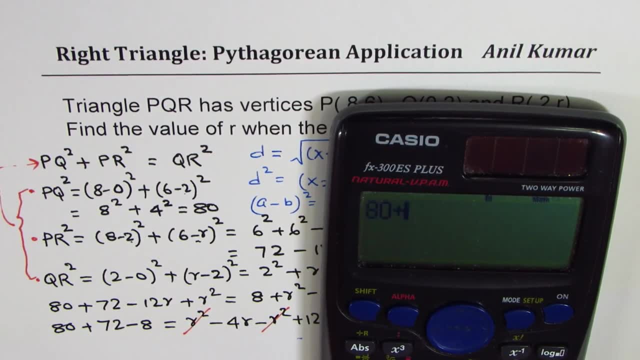 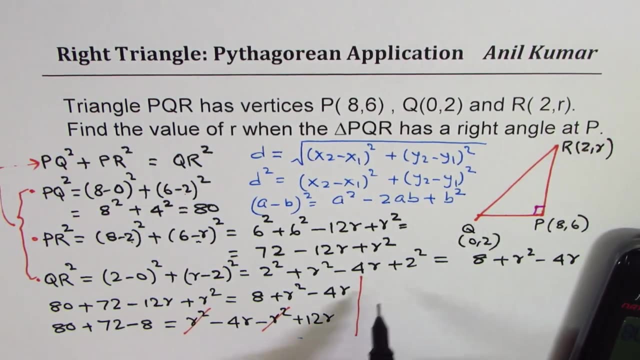 square is 0.. So we have a linear equation. So we could write this as: let's calculate the left side, which is 80 plus 72 minus 8 equals to 144.. And let's write down here: So we have 144,. 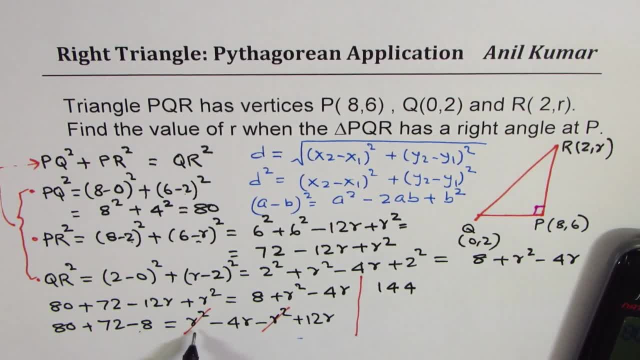 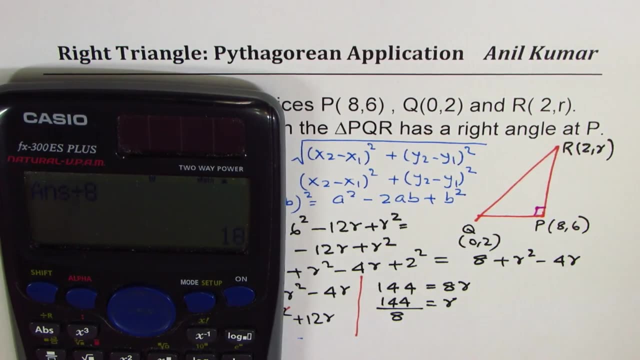 80 plus 72, minus 8 is equal to minus 4 plus 12,, which is 8, right, So 8R. So that gives you the value of R as 144 divided by 8.. So I'm going to divide this by 8 to get the answer. 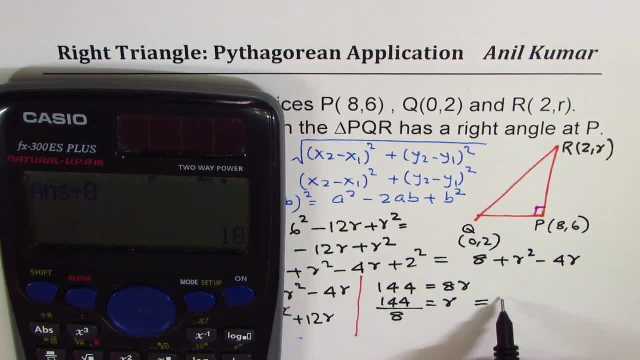 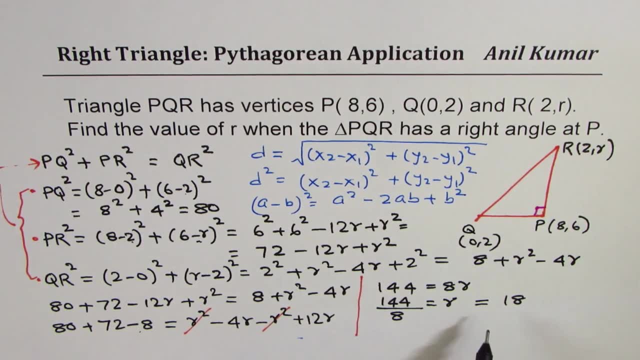 So that gives us the value of R as 18, right? So R is 18 for us. So that is how we could actually solve this particular equation, right? So I hope the concept is clear. So R is 18.. Feel free to write your comments and share your views And, if you,